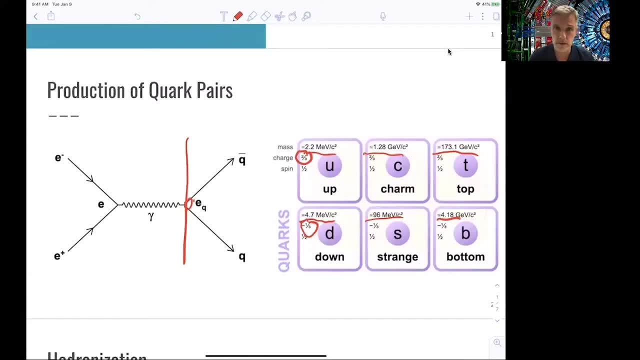 the couplings one. So this might cause some difficulties later on. OK, so now we want to produce an up quark and an anti-up quark in these collisions. What happens? So in our collisions then we produce those particles. So let's say there's an up. 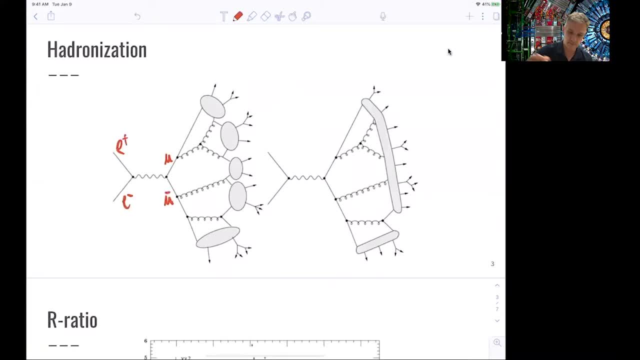 quark and an anti-up here and then a plus, a minus collision. Those quarks only live for a very short time or travel a very short distance in space- about 10 to the minus 15 meters- And then they start to pull in out of the vacuum. gluons and quarks and anti-quark. 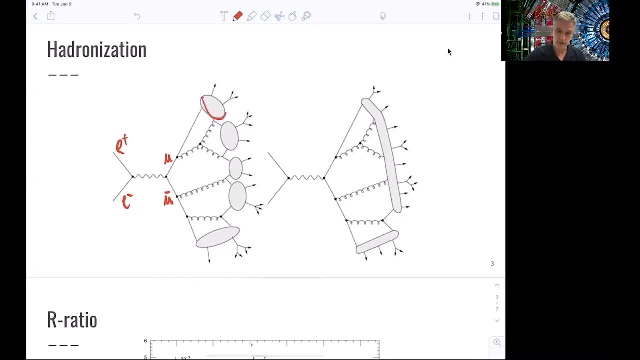 pairs And then form into the actual hadrons after some time. And those two pictures here. they look very much the same. The difference is the way we treat the hadronization, the actual fact of forming hadrons. In this first picture we 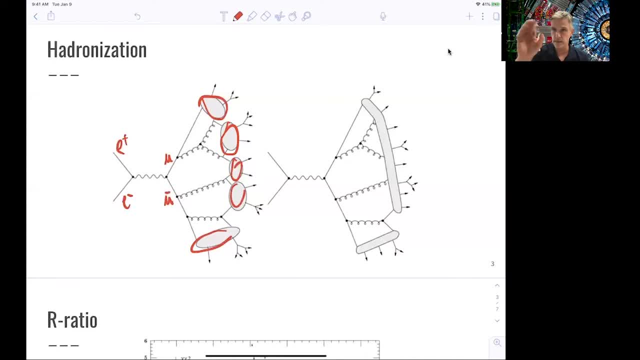 are thinking about clustering energy particles together and that way form hadrons In this picture here we connect them with so-called strings And those are two different ways to model and model the production of hadrons. Remember, when we look at this process, here we are looking 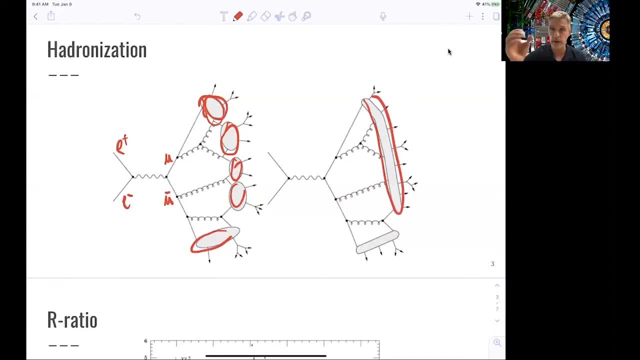 at very low-energy kind of or lower-energy kind of phenomena And at lower energies. the strength of the strong interaction, the strength of Q3D, is the coupling is in the order of 1, or can be larger than 1. So perturbation theory is not possible. That's why we need 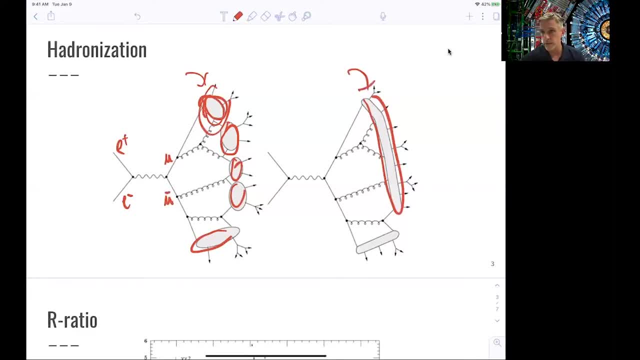 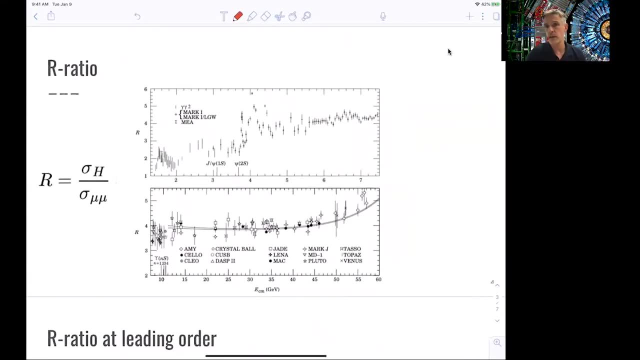 specific models. This is all I want to say at this point. We can now move on to the next slide, And we can come back to this discussion later on. What I actually want to discuss is what we can learn out of measuring. cross section of. 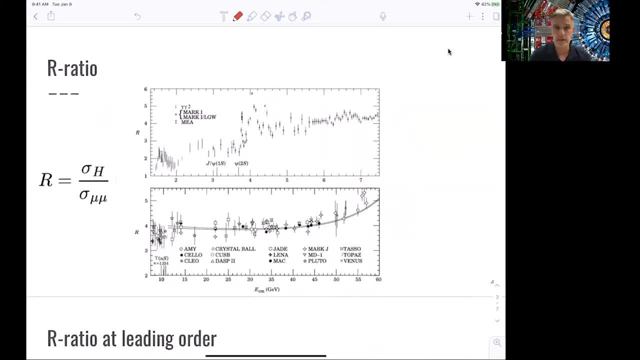 hadron production, For example, by comparing directly. the cross section of quark-anti-quark wave production is a cross section we just calculated for muon-anti-muon production And experimental results are given here. So you see, as a function of energy here from: 1 GeV to 7 GeV center of motion. And we get that. we get a matching load of energy, what we generate. So we get up to 40 degrees And then we calculate the positive and negative charge in the back And we calculate the mean and negative charge. So we just get a matching. 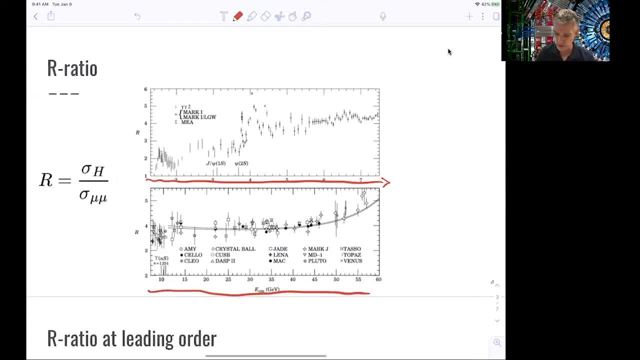 of in this form, And we are going again now by using this to get a better idea of zero of mass energy and then the lower plot just continuing from about 10 to 60 GeV. What you see here is that there is a rich structure. 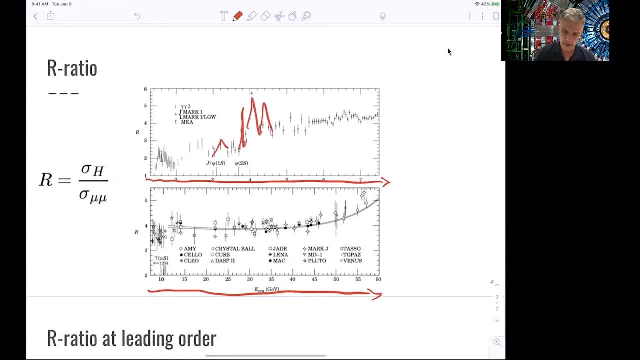 So you see those resonance here And you also see that there seem to be some sort of increase in the value of this ratio. So how can we now understand this? At leading order, we can just write this down. We just calculated the cross-section. 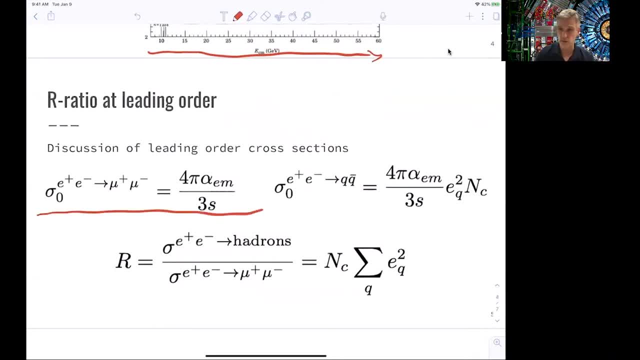 for electron-neuron scattering or for electron-neuron production, And we can write this very same cross-section at leading order for quark-antiquark production. What we find as differences is the coupling itself. Here we have to use the charge of the quarks. 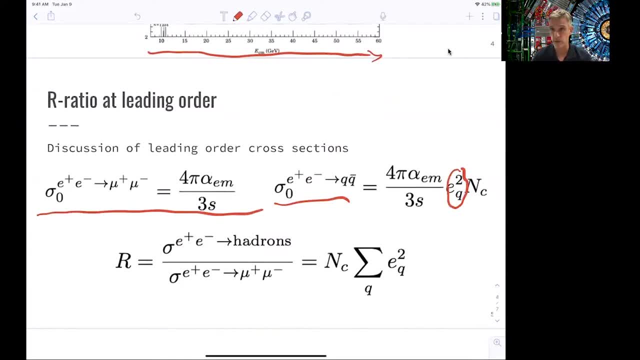 and not the charge of the electron. So there's an additional factor here: 1 third or 2 thirds squared, And then there is The number of possible quark pairs which are available, And that depends on the number of colors. Remember, each quark appears with three different colors. 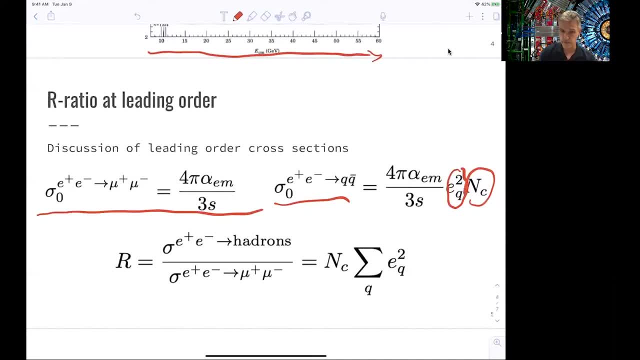 So we have to account for this factor, All right. And then we build the ratio And the ratio. everything just cancels out. Great. So we have just the number of colors times the sum of the charges squared of the quarks available. 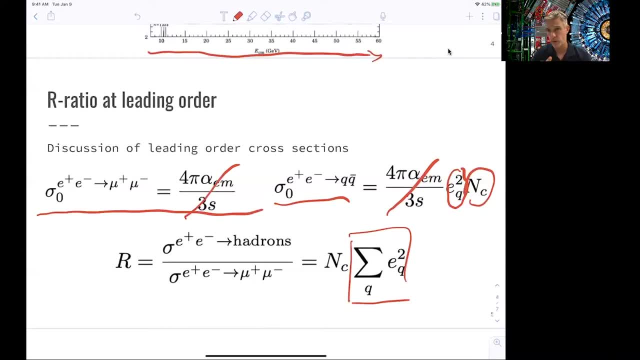 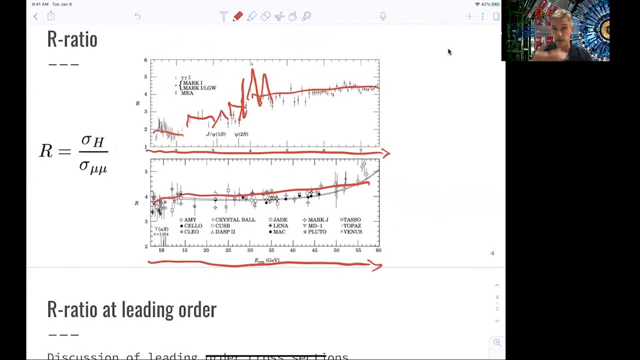 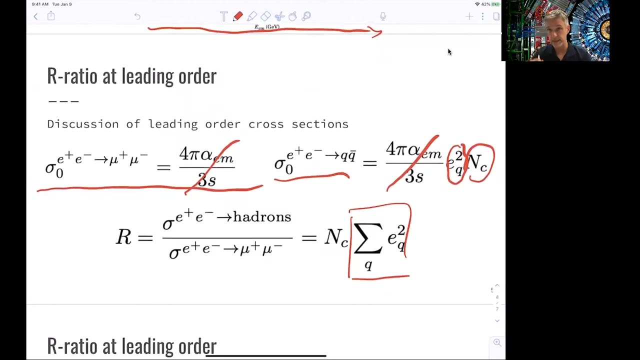 What do I mean by the quarks available As we go from From lower energies to higher energies? in this plot here, The kinematics, the energy is sufficient to produce particles based on the masses available. So we find that this explains the step function. 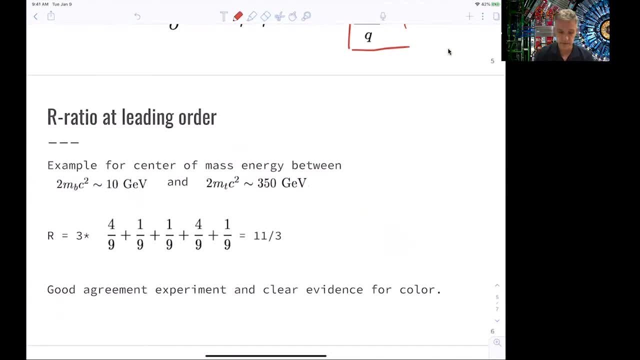 Let's look at a specific example. So if we look at center of mass energies which are larger than 2 times the mass of the bottom quark and maybe lower than 2 times the mass of the top quark, we are in this specific region. 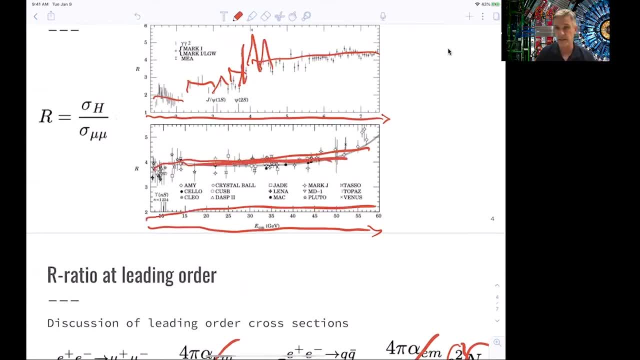 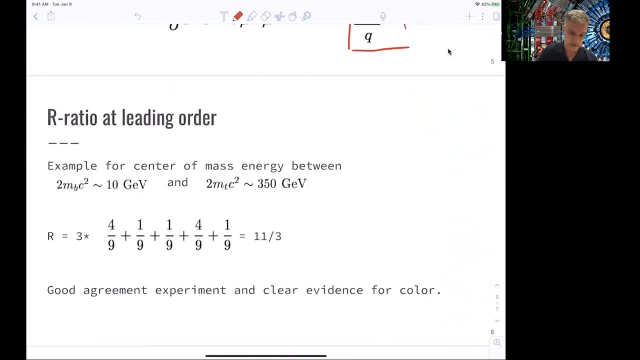 Here, And you see this is almost flat And the number we get is almost 4.. OK, What we get from this leading order calculation is 3 times 4 over 9 for our up quark 1 over 9 for down. 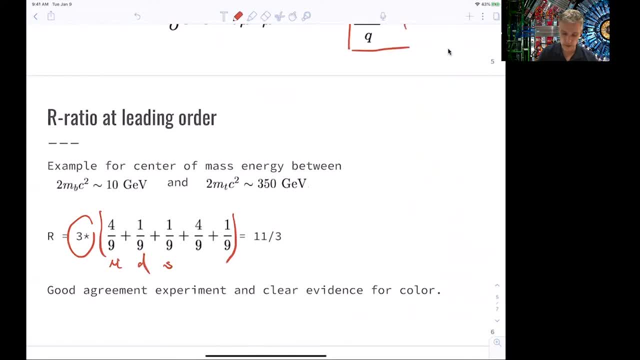 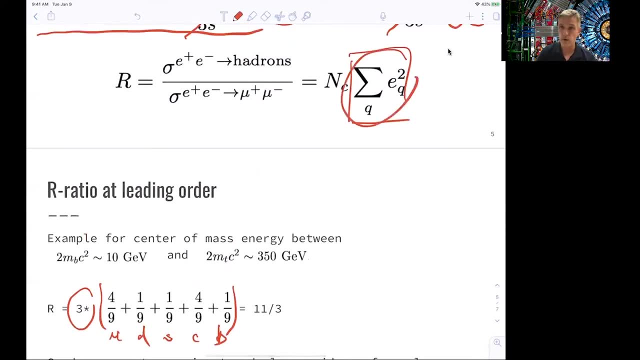 1 over 9 for charm, strange, 4 over 9 for charm and 1 over 9 for our bottom quark. OK, So we built the sum here For all quarks which are kinematically available And as an answer we get 11 over 3.. 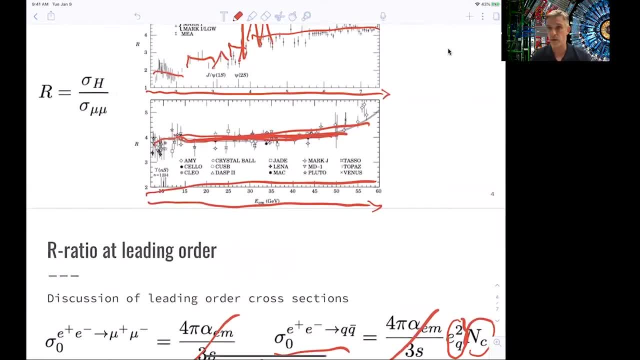 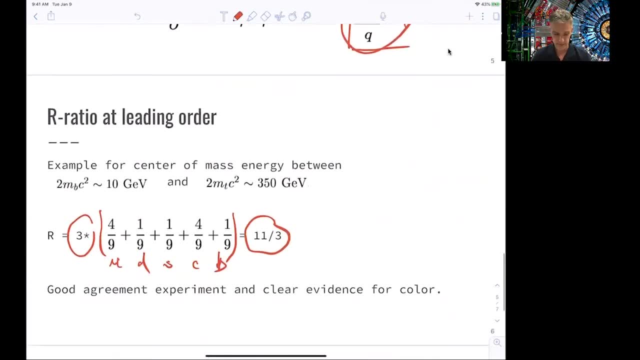 So this is in very good agreement, a leading order, a very good agreement with the experimental results: 11 over 3 is almost 4.. Excellent. So this is clear indication, experimental indication, that this color factor here is a real thing. 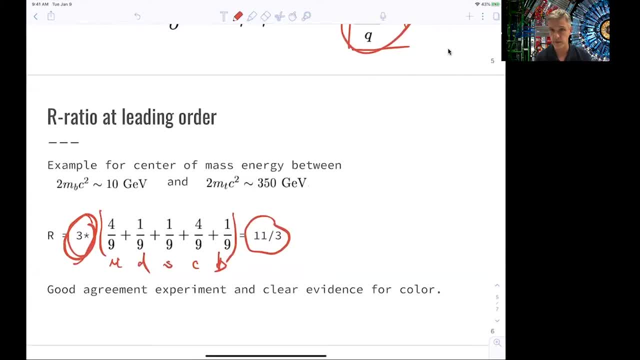 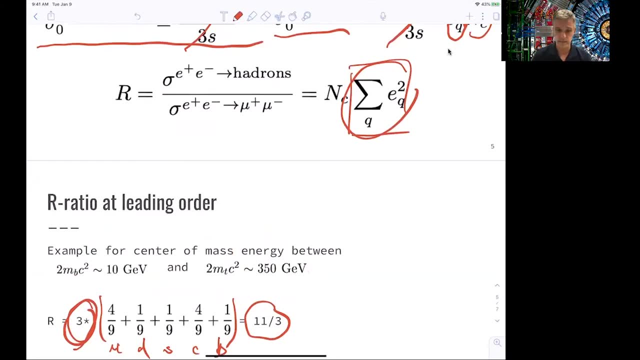 There seem to be three up quarks, three down quarks, three charm quarks and so on. OK, And we also see that this leading order effect, here the leading order calculation, is already very precise, And the reason for this is that this process here 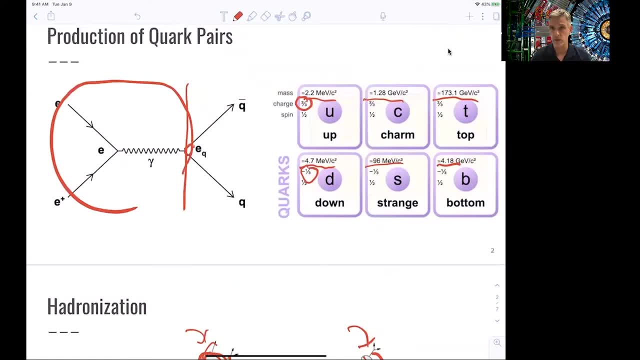 is a QED process, So the production cross-section is a QED process, as we discussed. So now, why do I actually have this as part of our Q3D introduction? First, we learned about the color factor here, OK, And second, 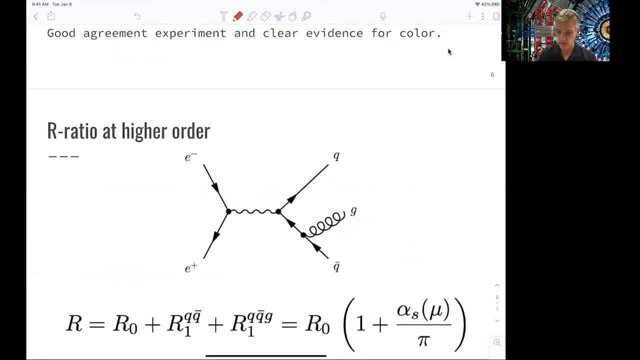 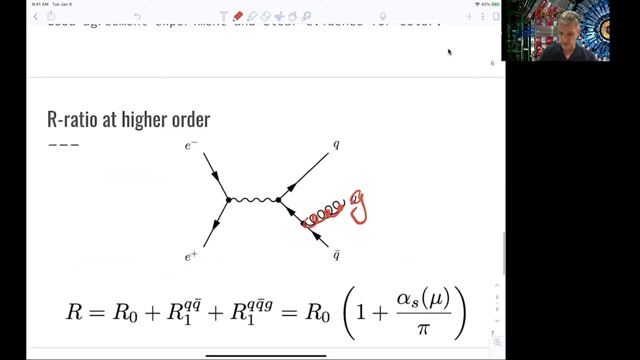 There is indeed corrections, And one of the correction is the one where you actually produce a real gluon in the final state And those corrections can be calculated. If you go to higher order, you get a correction from this radiated gluon. 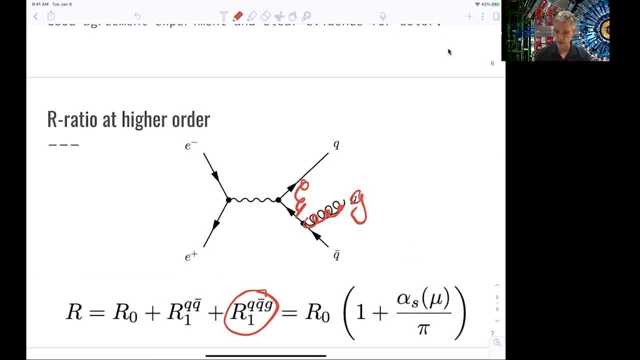 You also get corrections which look like this, vertex corrections, And you find that the correction here to R is about 1 plus alpha s At a specific scale over pi. Now, at a reasonable scale, this is then about 0.1.. 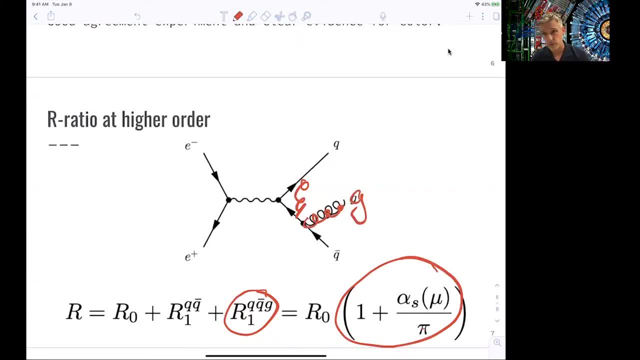 It's the value of alpha s And pi is 3.14.. And so you get about a few percent- 3%- correction to the R value. Great, Why is this so important? when it's a small correction, It's a percent or few percent level correction. 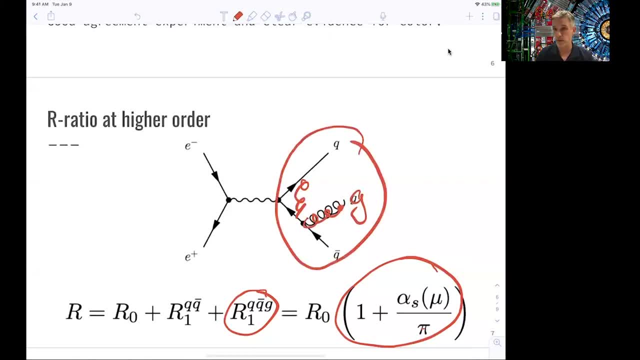 What is really important is that this processing can be used in order to demonstrate The existence of gluons, And so gluons have been discovered this way, And the way this was done is by producing E plus E minus collisions and detecting three bunches of particles, two from the quarks. 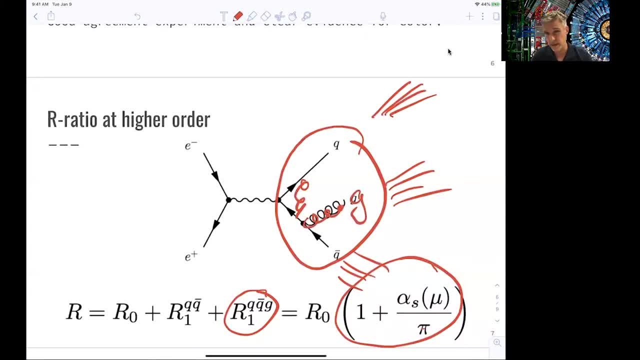 and one from the gluons And then to identify that this gluon here is actually a gluon and not some other particle. one can look at angular distributions, One can identify that this has been one particle, and so on. So there's a little bit.